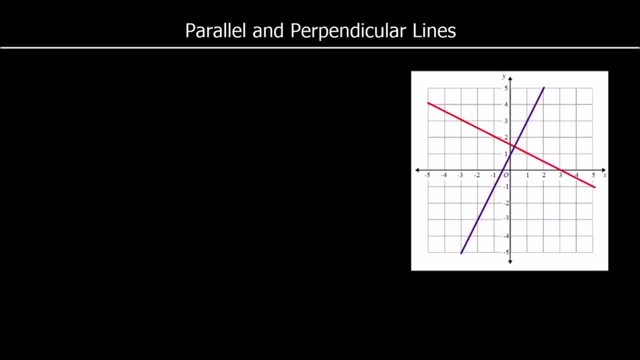 Parallel and perpendicular lines. Parallel lines have got the same gradient. They go in the same direction. So if we look at the purple line we can see for every one it goes across, it goes up two, Across one, up two, Across one up two. So we can say that the 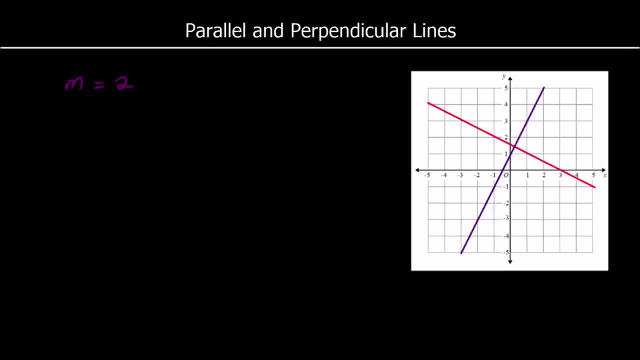 purple line has got a gradient of two And any other line with a gradient of two, no matter where it is on the graph, will be parallel. So these two purple lines are parallel. They've both got the same gradient. Perpendicular lines meet at a 90 degree angle. They meet. 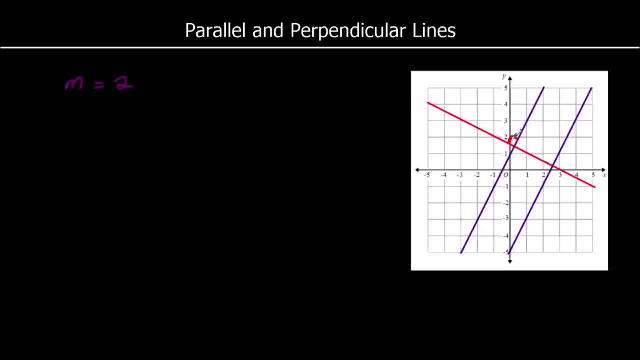 at a right angle. So there's a right angle in between the purple line and the red line, So they are perpendicular. The red line goes along two down one, Along two down one, Which means for every one it goes across it goes down by a half Across one down a half. 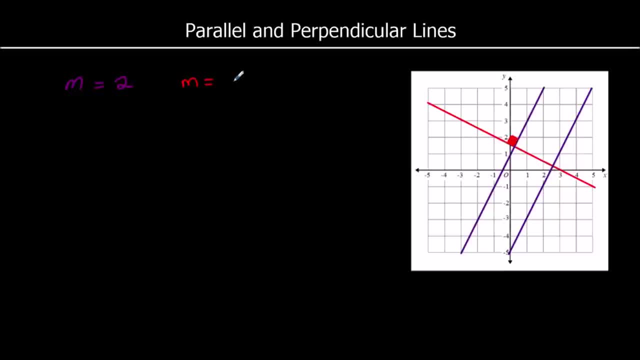 So the red line has got a gradient of minus a half. For every one it goes across it goes down by a half. There is a relationship between the two. There is a relationship between these two gradients. If you multiply them together, if you multiply together the gradients of two perpendicular lines, you will always get 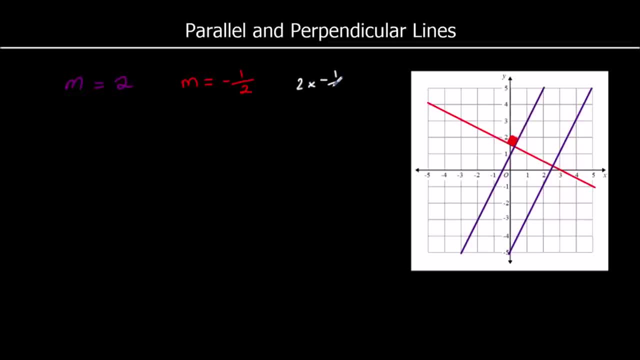 negative one. So two times minus a half is negative one. Or what you could say is that one is the negative reciprocal of the other one. So if one perpendicular line is positive, the other one would always be negative And the gradients are flipped over. So a gradient of two for one means the other one's got a. 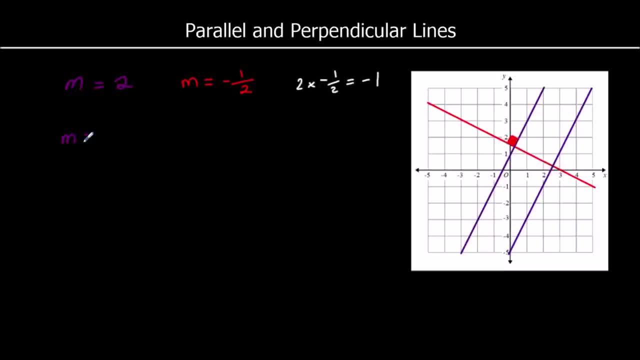 minus a half. If one had a gradient of four, its perpendicular line would be negative And the reciprocal of four, which is one over four. If a line had a gradient of three, the perpendicular line would have a gradient of. it would be. 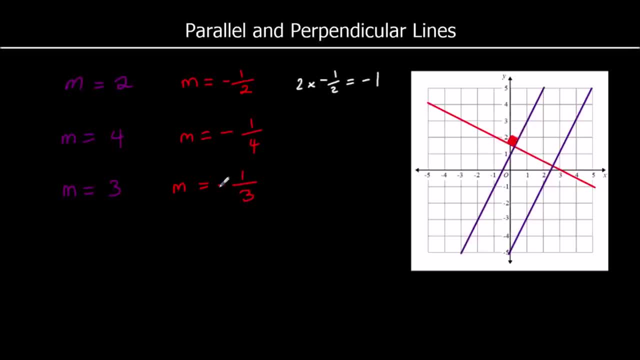 negative and it would be one third So negative, reciprocal. If we had five over two for one of them, the other one would be negative and two fifths So negative and flipped over. If one had a gradient of minus four fifths, its perpendicular line would have a gradient. 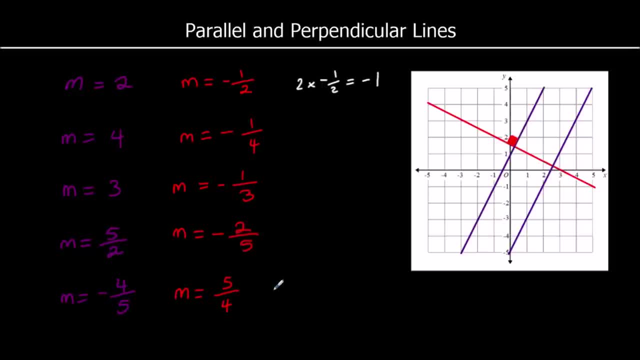 of positive five over four. So we can either say that the gradients of two perpendicular lines multiply to make negative one, Or that one of them is the negative reciprocal, Or that one of them is the negative reciprocal of the other one. Let's look at some questions. 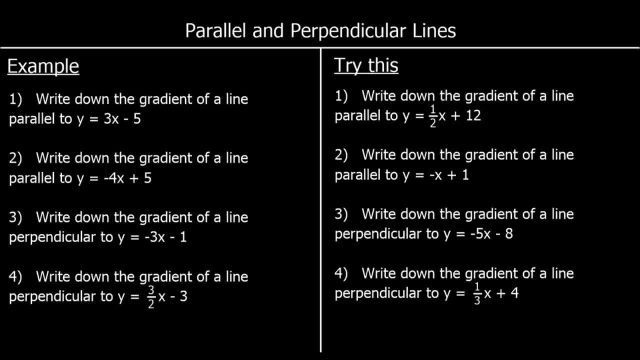 So the first one says: write down: the gradient of a line parallel to y equals three x minus five. So the equation of a straight line is in the form: y equals m x plus c, where m is the gradient And c is the y intercept. 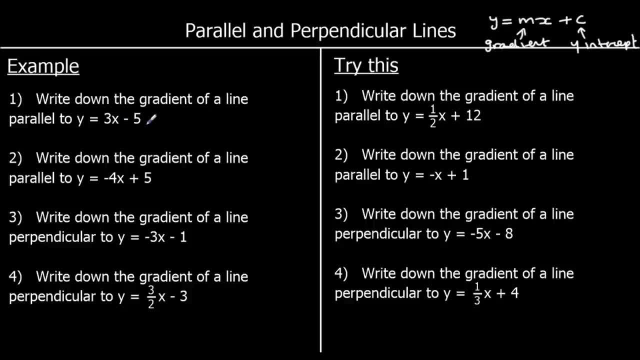 So the gradient of y equals three. x minus five is three, And a parallel line will have the same gradient. So any parallel line will have a gradient of three. For the second one, write down: the gradient of a line parallel to y equals minus four x plus five. 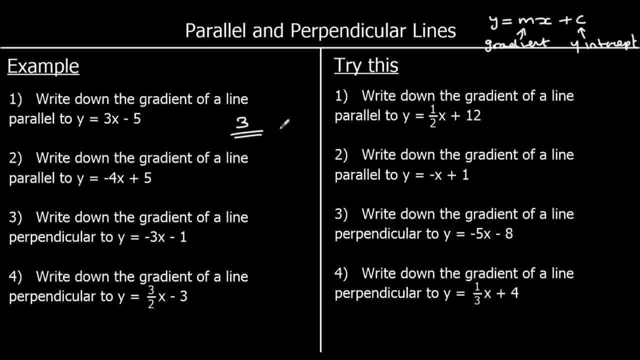 The gradient of this line is minus four, negative four, And any parallel line will have the same gradient. Question three: Write down the gradient of a line perpendicular to y equals minus three x minus one. So the perpendicular gradient is going to be the negative reciprocal. 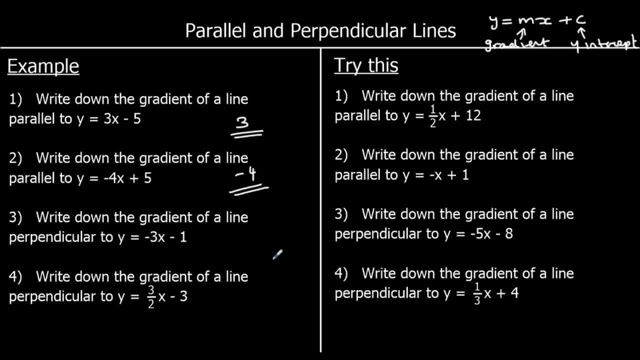 So the gradient of this line is negative three. So the perpendicular gradient is going to be positive one third. So if one of the lines has got a negative gradient, the other one's got a positive gradient And the reciprocal of three is one third. 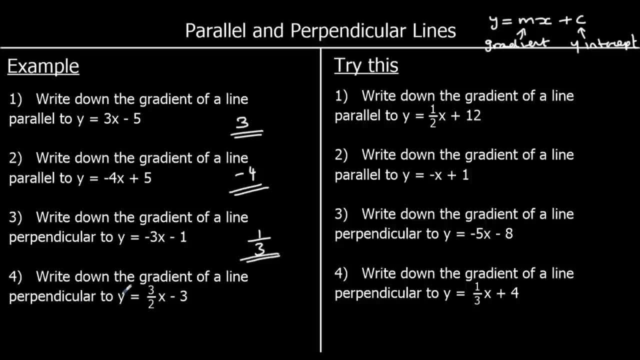 Write down the gradient of a line perpendicular to y equals three over two, x minus three. So again negative. reciprocal of three over two. So it's going to be negative. And three over two flipped over is two thirds. Okay, four, for you to try. 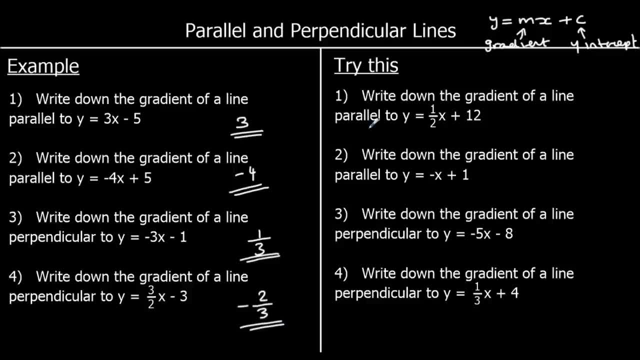 So give them a go. So parallel to y equals a half x plus twelve. Any parallel line's got the same gradient And that is one half. Write down: the gradient of a line parallel to y equals minus x Plus one. So the gradient of this line is negative one. 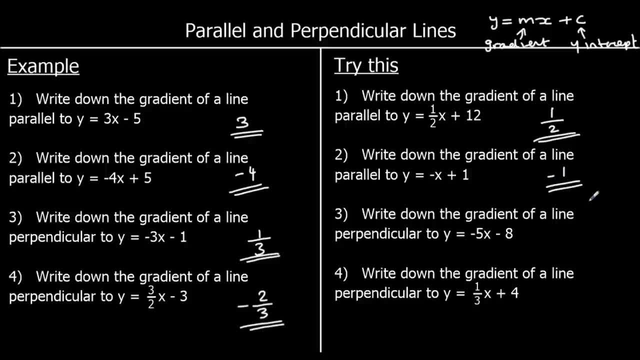 And any line parallel will have the same gradient Perpendicular to y equals minus five. x minus eight. We want the negative reciprocal of negative five, So it's going to be positive one fifth. The last one, y, equals one third x plus four. 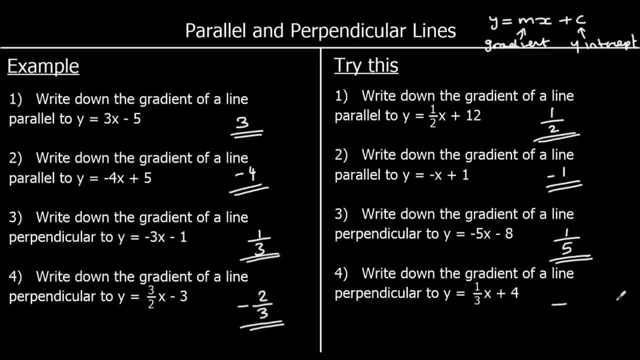 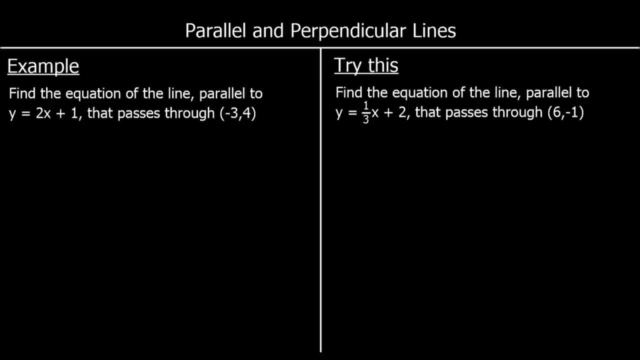 This one's positive, So the other one's going to be negative, And the reciprocal of one third is three. Okay, a different example. Find the equation of the line parallel to y equals two x plus one. So if it's parallel to y equals two x plus one, it must have a gradient of two. 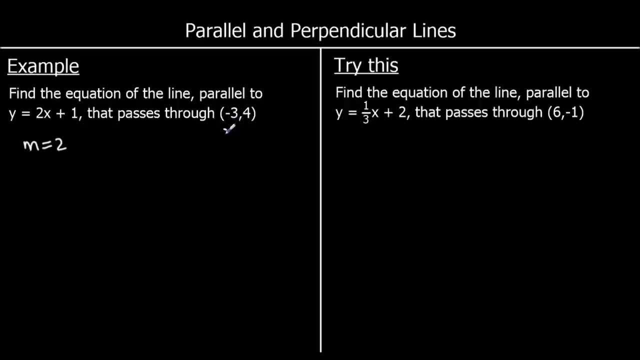 That passes through the point minus three four. So the equation of a line is in the form: y equals m x plus c. We know the gradient's going to be two, So it's going to be y equals two x plus c. To find c we're going to substitute in these coordinates: 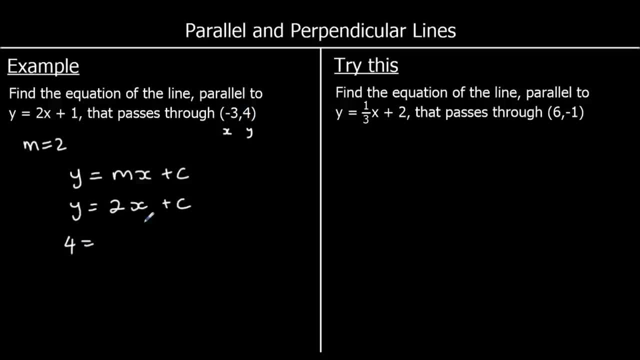 So y is going to be four And x negative three, Two negative threes and negative six And plus negative six to both sides to get c by itself. So c is ten. So we've got y equals two x plus ten. Okay, one for you to try. 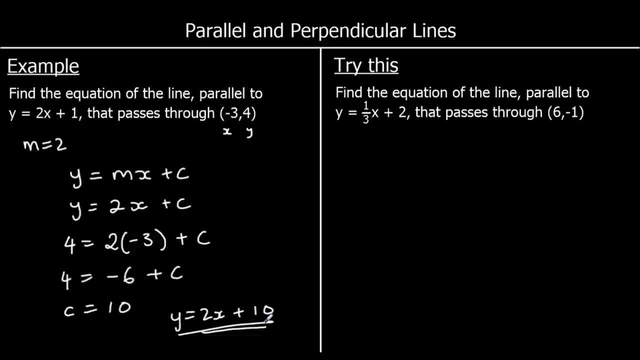 So give this one a go. Find the equation of the line: parallel to y equals one third x plus two. That passes through six minus one. So it's parallel, So the same gradient. So m is one third. So we've got y equals one third x plus c. 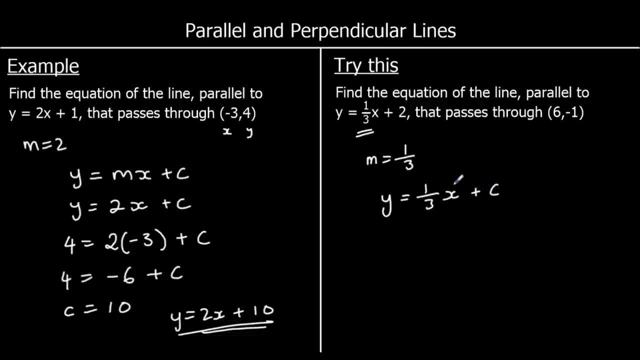 To find c, we're going to use the coordinates we've been given, So x and y, Which means we've got minus one, equals one third Times six plus c. One third of six is two. Take away two from both sides. 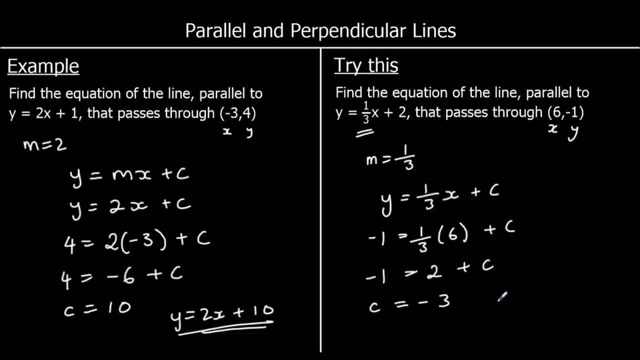 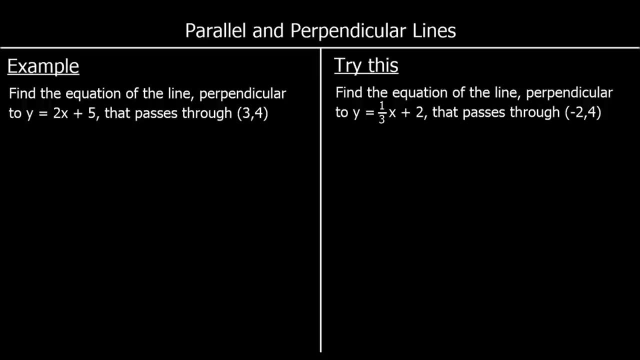 So we get: c is negative three. So we've got y equals one third x minus three. Another example: Find the equation of the line perpendicular to y equals two x plus five. That passes through three, four. So we want the perpendicular gradient this time. 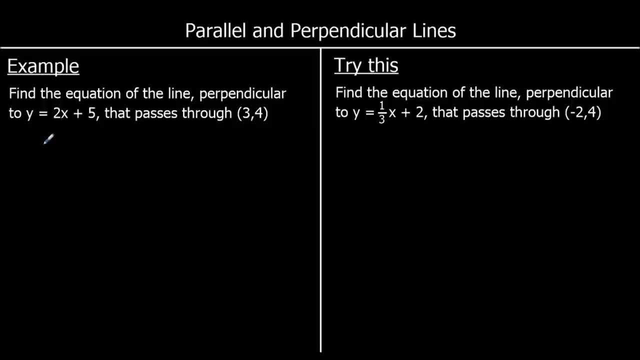 So the negative reciprocal of two- So flip it over- And minus The negative reciprocal of two is minus a half. So we've got y equals minus a half, x plus c. To find c we're going to use our coordinates of the point. 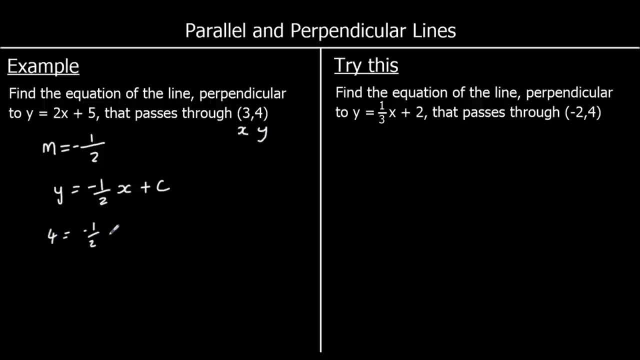 So it's going to be four equals minus a half times three, plus c. Minus a half times three is minus one and a half, or minus three over two, And to get c by itself, we're going to plus three over two or one and a half to both sides. 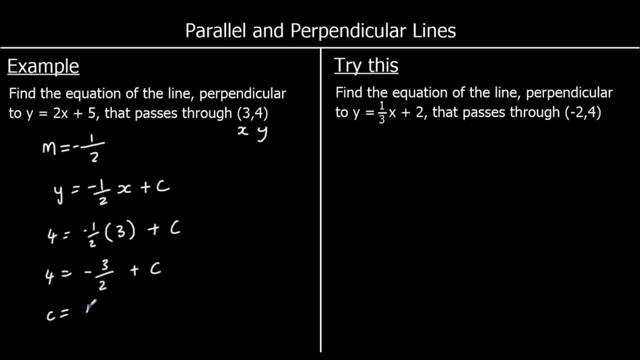 So c is going to be five and a half, Or 11 over two. So we've got y equals minus a half x plus 11 over two. Okay, One for you to try, So give it a go. So we want the perpendicular gradient. 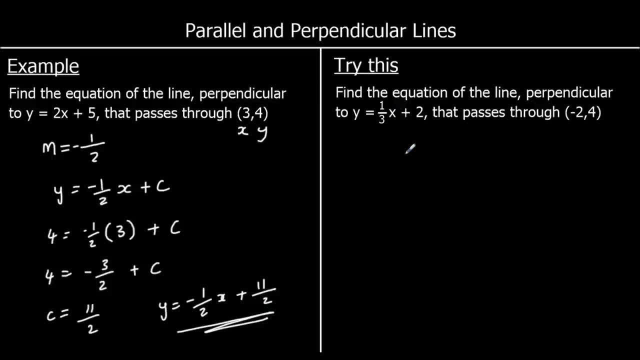 So it's one third. So the negative reciprocal of one third is minus three. So flip the minus Minus three, So we've got y equals minus three, x plus c. We've got a set of coordinates that we can use to find c. 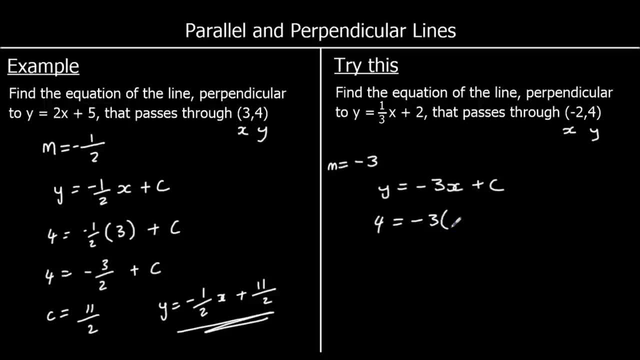 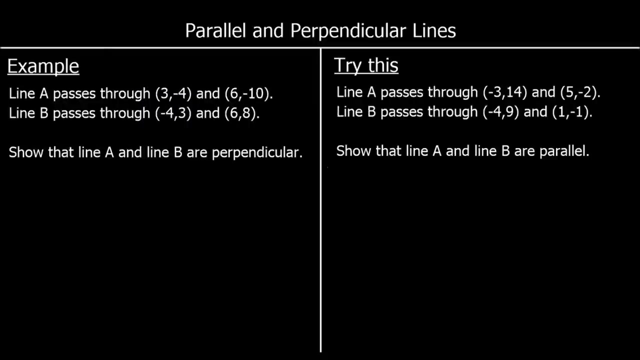 So y is four And x is negative two. So negative three times negative two is six And take six away from both sides, Take six away from both sides to get c by itself. So c is negative two. So y is minus three, x minus two. 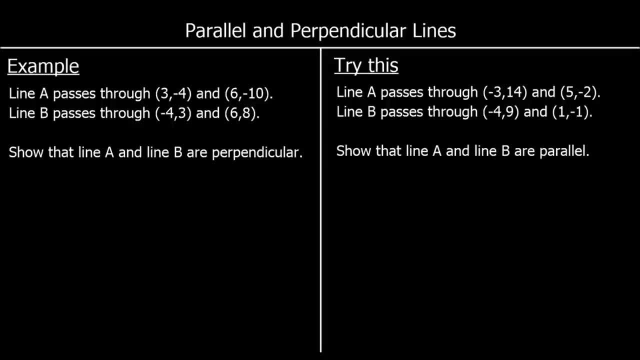 One more example We've got: line a passes through three negative four and six negative ten. Line b passes through negative four. three and six. eight Show that line a and line b are perpendicular. So we're going to work out the gradient of line a and the gradient of line b. 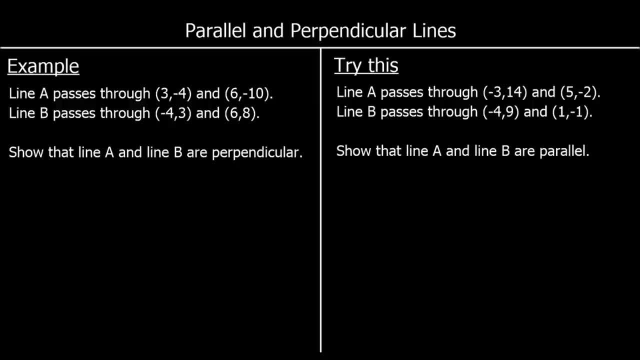 And then show that they multiply to make negative one, Or show that one gradient is a negative reciprocal of the other gradient. We will work out the gradient By working out the change in y Divided by the change in x, And we can use the formula. 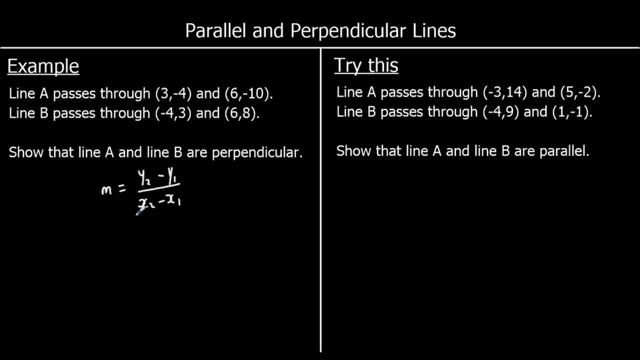 M is y two minus y one, over x two minus x one, So the change in the y's Divided by the change in the x. So we'll label the points x one, y one, X two, y two For both of the lines. 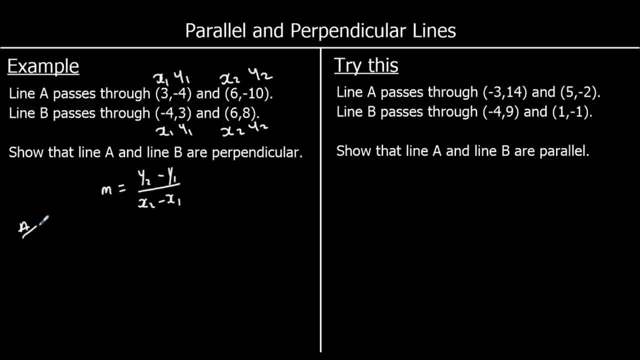 And then we can just substitute them in. So for line a The gradient Is y two minus y one, So negative ten Minus negative four. Over x two minus x one, Six minus three. So to simplify that we've got. 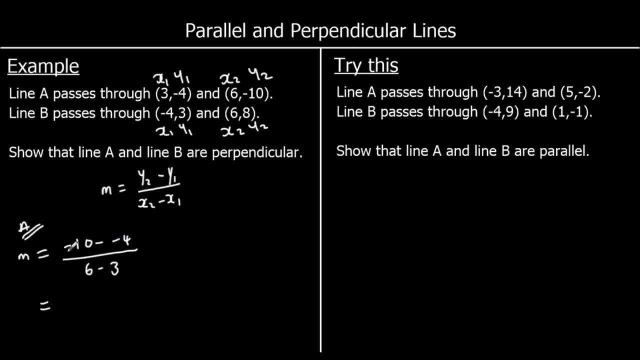 Negative ten. take away minus four, Which is the same as negative ten plus four, So negative six Over six minus three, Which is three, And six over three is two And it's a negative divided by a positive, So it's negative two. 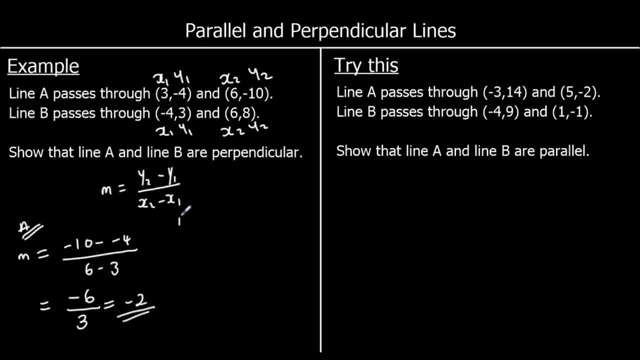 So a has got a gradient of negative two. For b The gradient is the change in the y's Y two minus y, one, Eight minus three, Over the change in the x's Six minus negative four. So eight minus three is five. 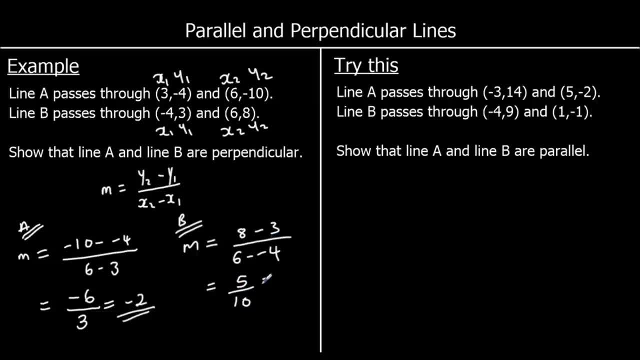 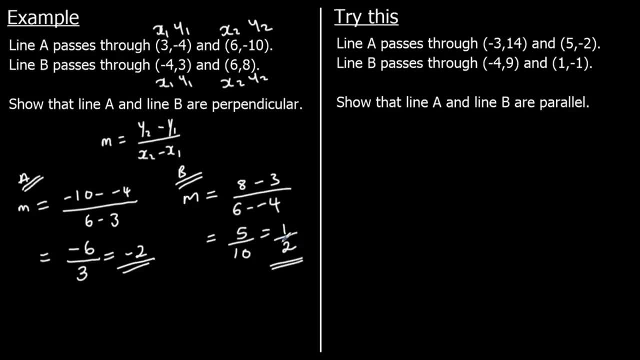 Six plus four is ten, So that's got a gradient of one half. So we can See by these two gradients They are Perpendicular Because they multiply To make negative one, Or we could say that one is a negative reciprocal. 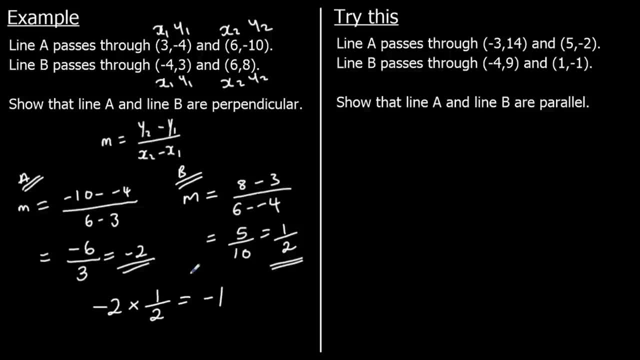 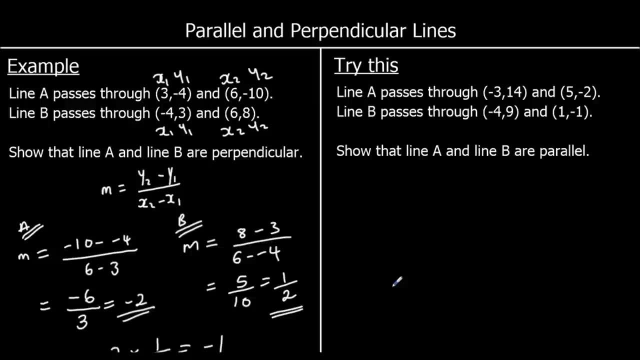 Of the other. Okay, One for you to try. So pause the video And give it a go. We've got. line a passes Through negative three, fourteen And five negative two. Line b passes Through negative four, nine And one negative one. 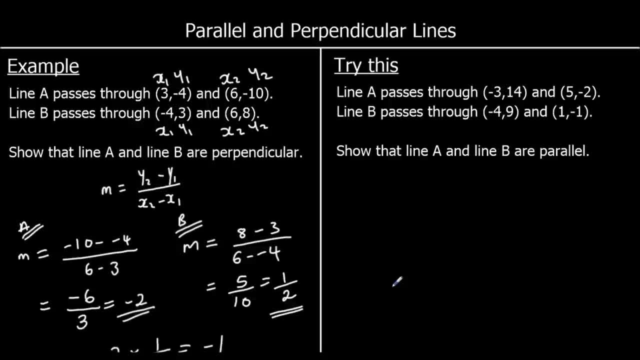 And we are showing they are parallel this time, So they will have the same gradients. So we are going to work out the gradient of both lines By doing the change in y Over the change in x, So we have x one, y one. 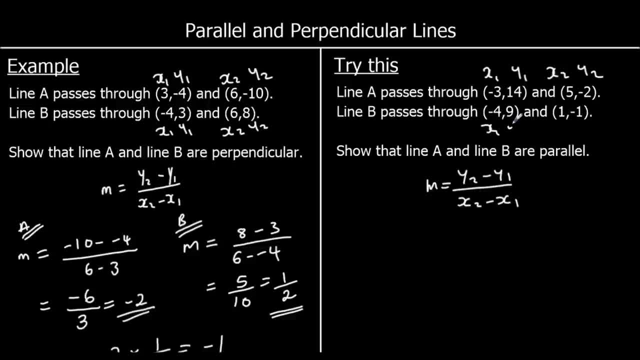 X two, y two For both lines. So for a The gradient is y two minus y one, Which is negative two minus fourteen, Over x two minus x one, Which is five. take away Negative three, So we have got Negative two take away fourteen. 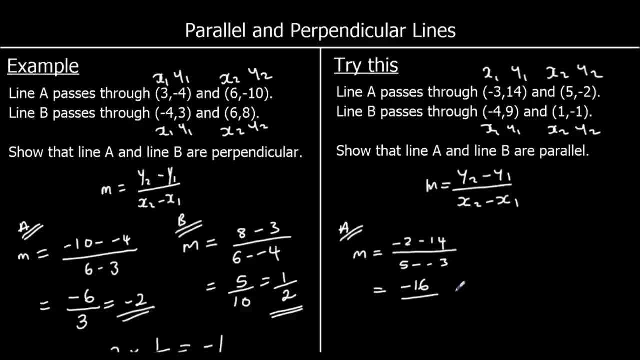 Which is negative. sixteen Over five plus three, Which is eight, We have got a negative divided by a positive, Which will be negative, And sixteen over eight is two. So a has got a gradient of negative, two, B The gradient. 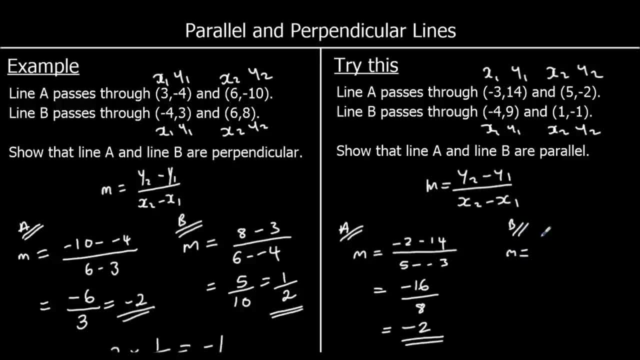 Is y two minus y one, Which is negative one Minus nine Over x. two minus x one, Which is one minus negative four. So negative one minus nine is negative ten. One plus four is five. Ten over five is two. 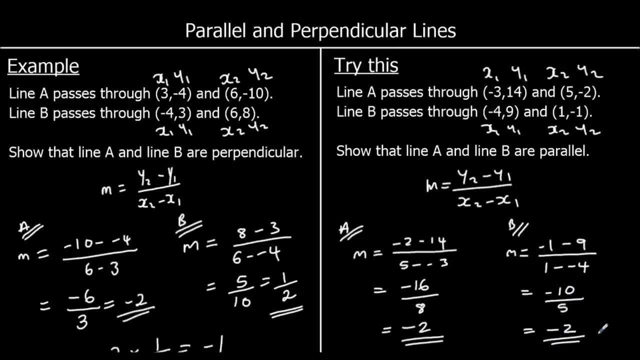 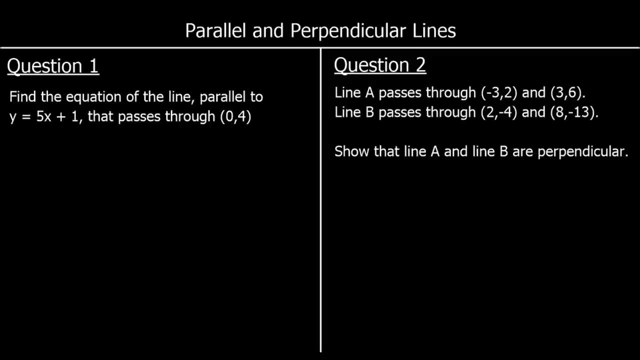 So negative ten over five Is negative two. So they have got the same gradient. Therefore they are parallel. To finish up, We have got two questions, So pause the video And give it a go. Question one: Find the equation of the line parallel. 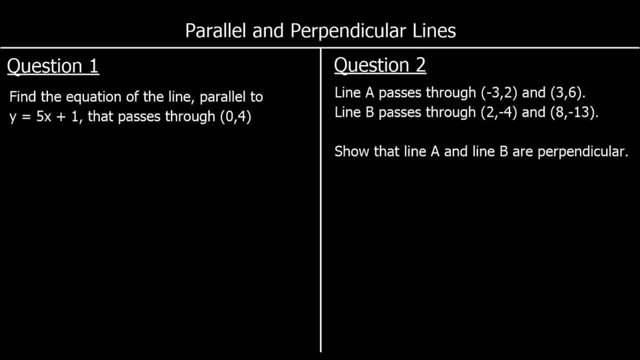 To y equals five x plus one That passes through zero four. So if it is parallel It has got the same gradient. So it must have a gradient of five. So it is y equals five x plus c And the y intercept. 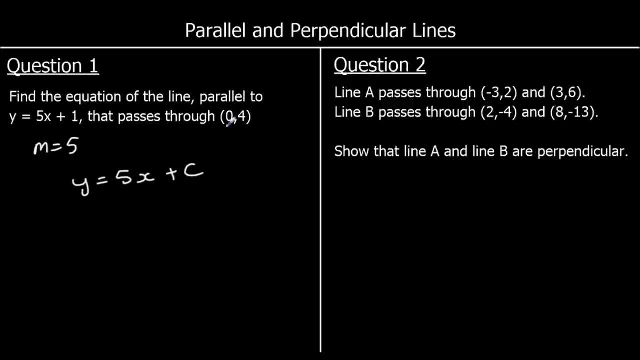 Is going to be four, So it goes through zero four. Zero four is the y intercept, So that means we have got y equals five x Plus four. For question two: Line a passes through negative three, two And three six. Line b passes through two negative four. 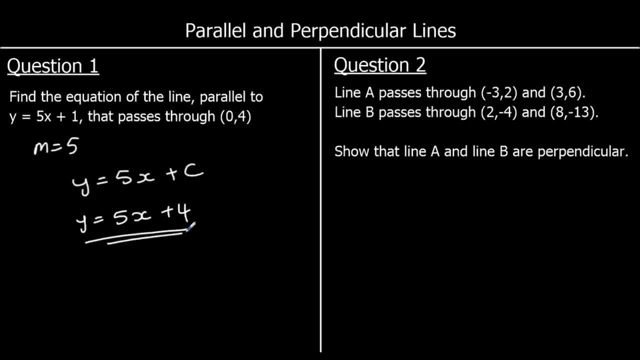 And eight negative thirteen Show that a and b are perpendicular. So we are going to work out the gradient of a And the gradient of b And then show that they multiply To make negative one. So to work out the gradient, We will do the change in y. 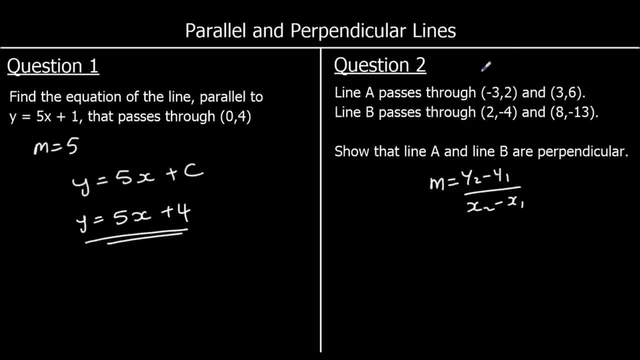 Over the change in x And we have x one, y one, X two, y two For both of our lines And substitute them in, So for a, The gradient is y two minus y one, Six minus two Over x two minus x one.